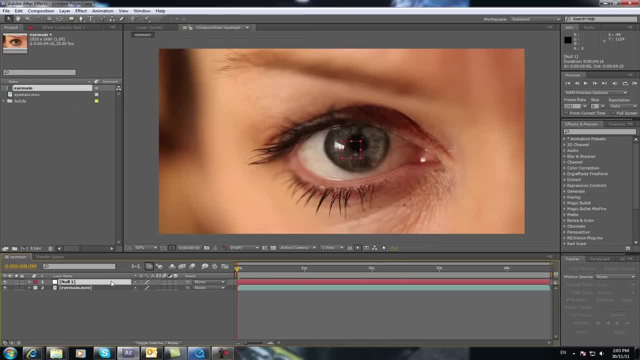 Select the Null Object and press Enter and call this one Tracking Data. You basically want to select your eye. This is your main footage. You need to track this footage because if you actually look at the footage, you see that it's actually moving around and what will happen is if you create the dilating pupil. 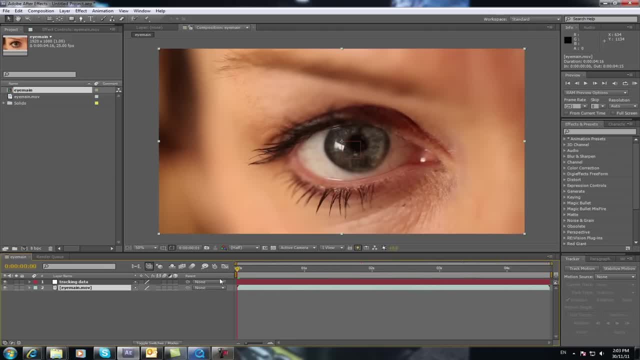 and your footage is moving around, it will be in the centre and you actually won't look realistic because it won't be matching the footage, It won't be stuck to the footage. So you go over here to your Track Motion option on the Tracker Controls and if you can't find that, 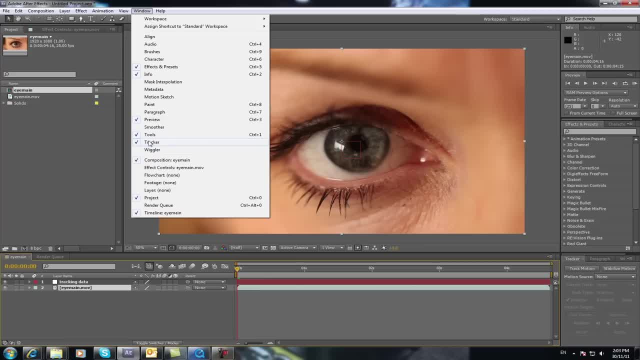 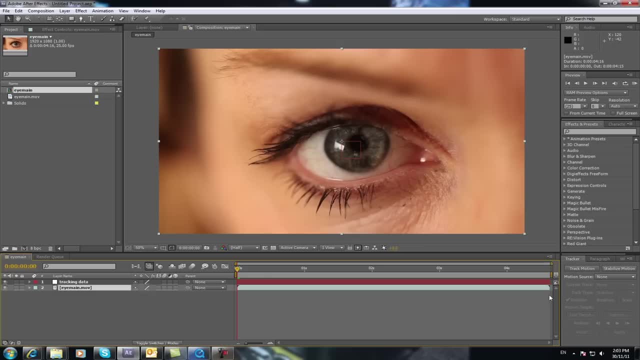 you just go Window and Tick, Tick the Tracker tab down here and it will pop up and you can use it. So you select your main footage. in my case it's called Eye Main. You go to Track Motion and we're going to track the rotation as well. 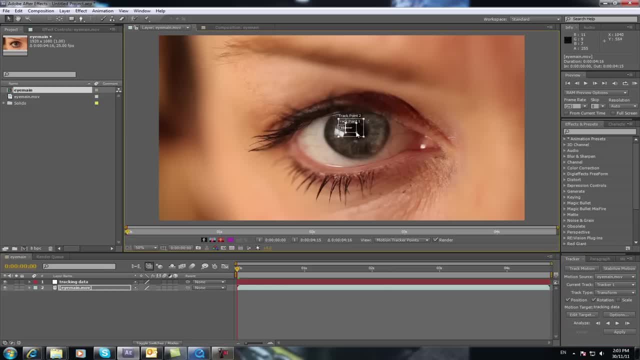 Now you want to pick. if you look here, you want to pick, say, the corner of the eye, because that doesn't really change much, and maybe the edge of the eyeball or something like that. I probably would go with the corner of your eye down here. 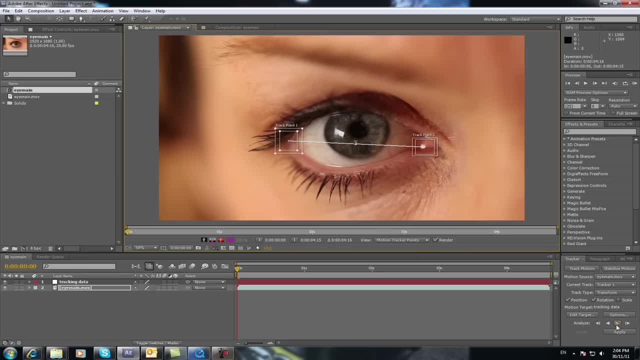 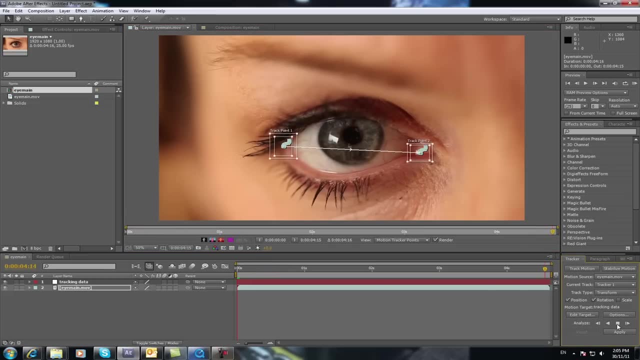 The whole idea is that you've selected that and now you go Analyse Forward down here. Okay, that was pretty good. If the tracking points move around too much whilst it's tracking, it means it's not in a secure spot, and that will make the effect look not quite as good. 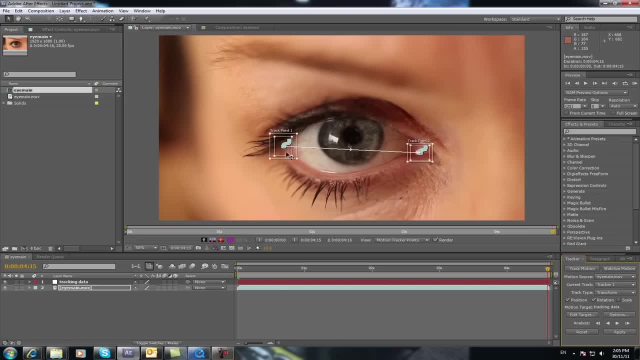 So you want to make sure that as you watch it being tracked, that sort of these squares stick in position. If they move around, go up and down too much outside where you began, then it won't work very well. You go Edit Target to make sure it's set to your tracking data, which is your null object. 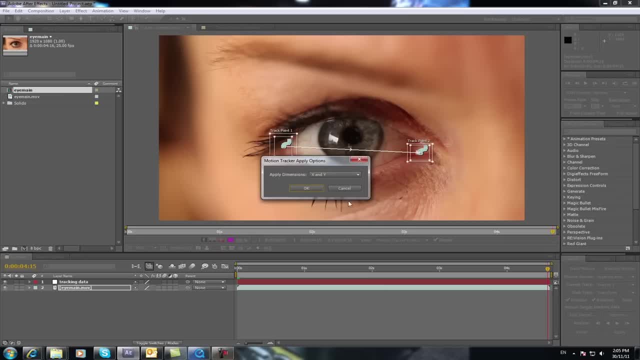 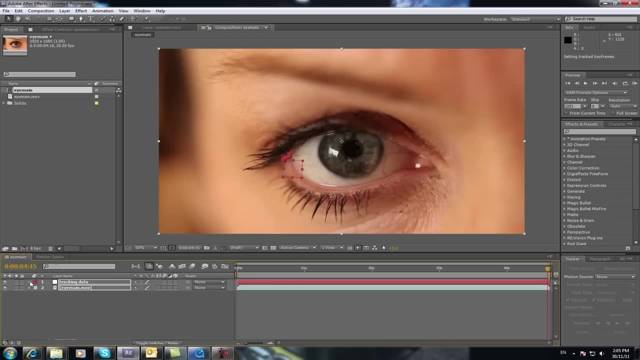 Go OK and select Apply. Select Apply to X and Y, Apply to X and Y and do OK. And now you'll see down the bottom here that all your data is actually attached. all that movement information is attached to the tracking data. null object. 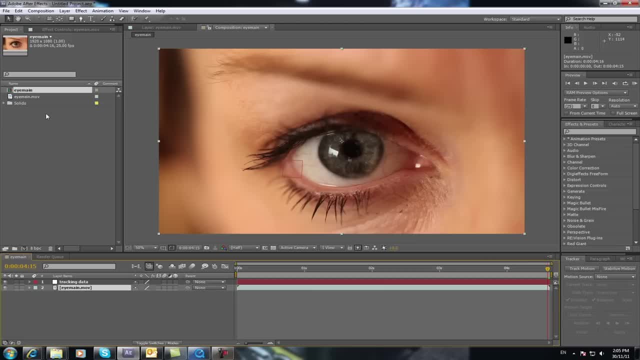 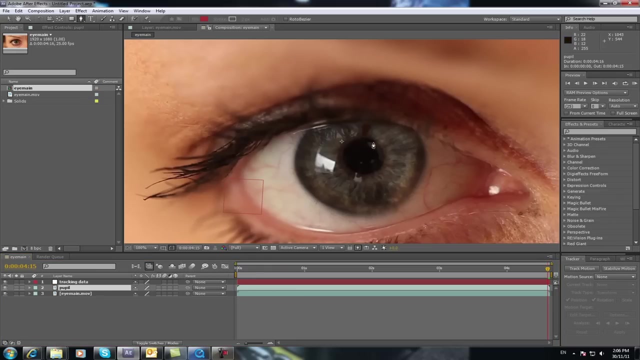 So now what you need to do is select Eye Main and do Edit, Duplicate And we're going to call this one, press Enter. Select it and press Enter, We're going to call this one Pupil. Okay, Now select it again and get your masking tool up here and draw a mask around just the pupil. 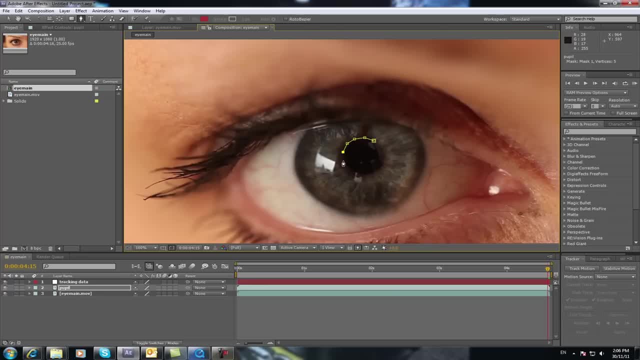 So it just doesn't have to be too perfect. You just want it as close as you can, just around the black area, like so, Like that. You want to select the arrow down here and select Masks, Select Masks again and Feather. I would make the Feather about 10.. 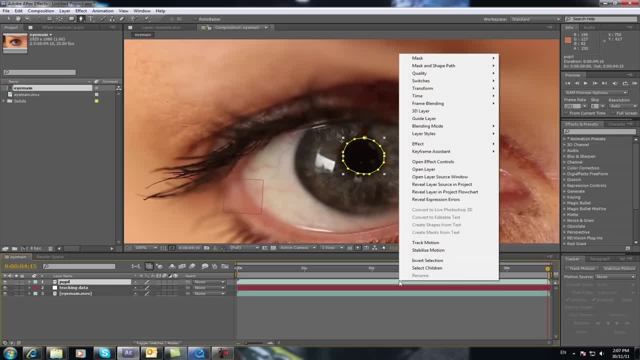 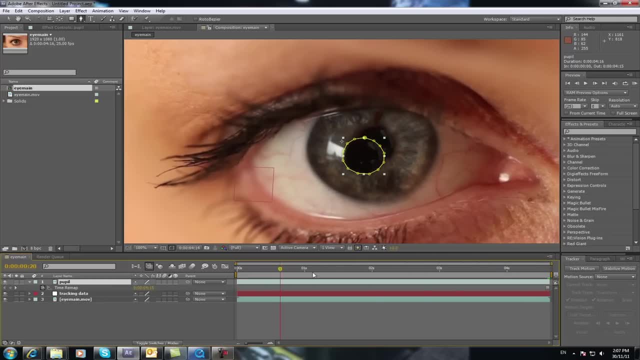 Okay, You've got the pupil. You've selected the pupil now. So now you want to do right click on the footage and go Time Freeze Frame- Okay. So now that pupil is the same old pupil it was before. It doesn't change, but it's not stuck to the eye, as you can tell. 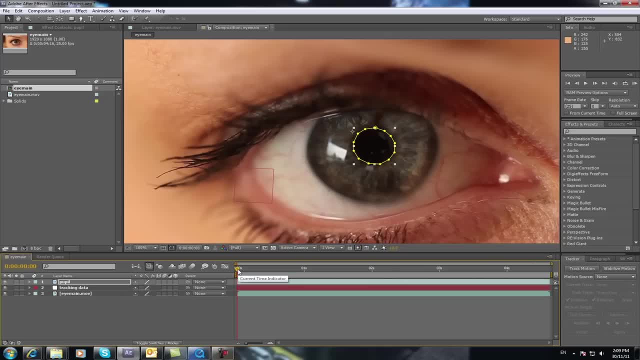 Okay, Now your pupil. you've done a freeze frame and you have your pupil sitting there like. so, As you can see, it doesn't move with your footage like it's supposed to. So now you want to get your make sure, when you go back to the start of your thing, that 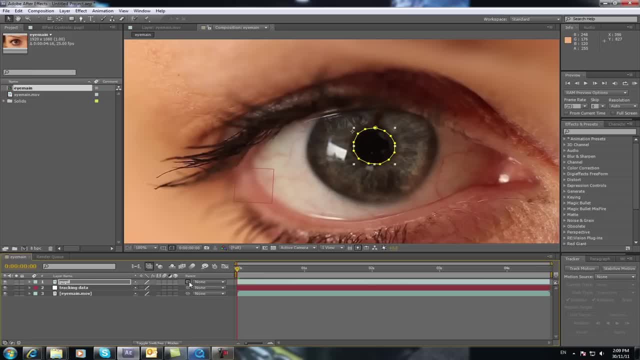 it is in position where you want it to be, Then you go pick where you can go, Pupil Tracking Data, like so. Now it's moving with your footage. As you can see, it's stuck to your footage, which is what you want. 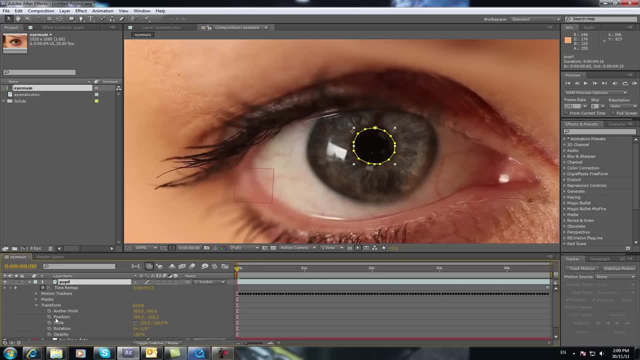 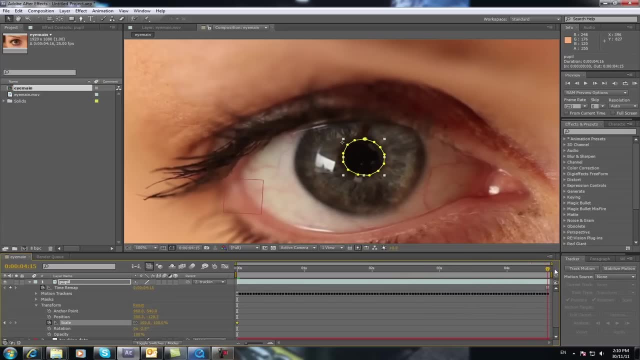 Okay, Now what you need to do is you need to go down to here and you need to select Scale. Now, at the start of this, you'll leave it at 100% and I suggest, maybe at the end of it, scroll to the end. hit the sorry at the start of the footage. hit the stopwatch to. 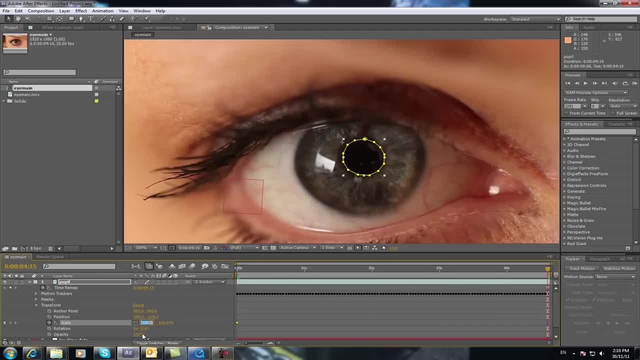 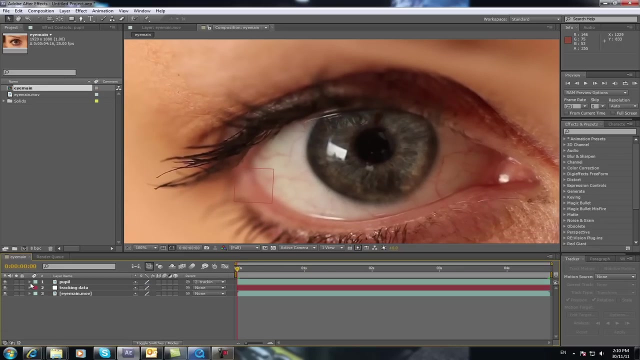 get a keyframe and then scroll all the way to the end and change that to say 300%, Change that to say 200%. As you can see, that's enlarging, but it's not enlarging with your eye. So you need to go to the pupil again and hit position stopwatch and at the end, at the